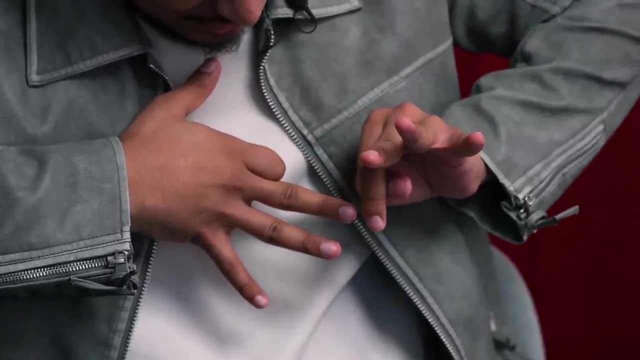 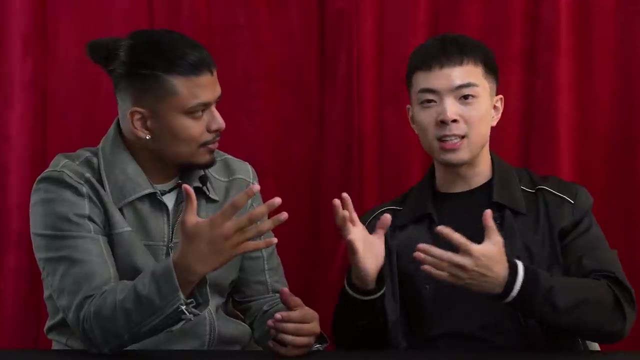 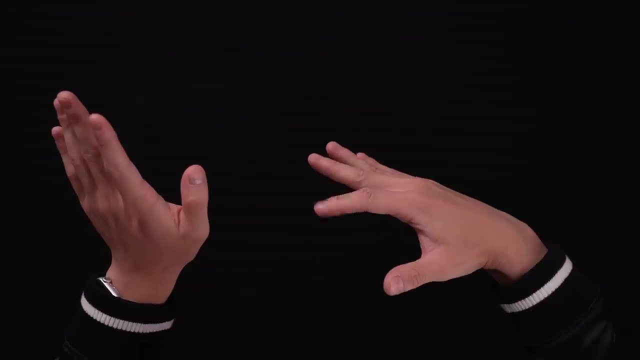 Okay, ready, There you go, Bro. What. I've seen this in preschool, but yours looks so much better, Let's do it. There's two things, okay. So your right hand is going to take your index finger and just bend like this Left hand is going to use your thumb and your thumb. 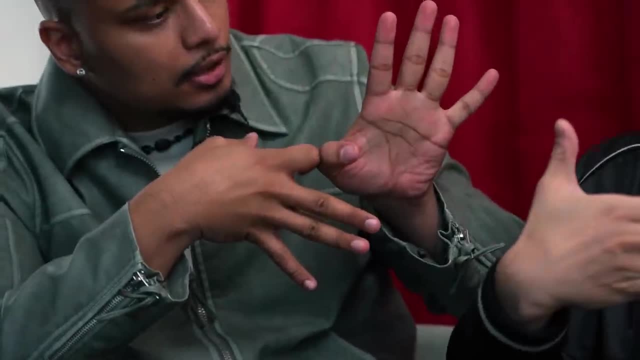 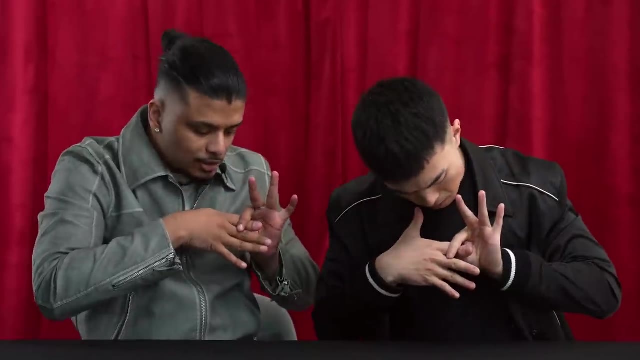 is going to bend like this, okay, All right. You're going to connect your knuckles together like this, Perfect. And then you're going to take your index finger here and you're going to cover that little gap, right, And the rest is really just your acting. 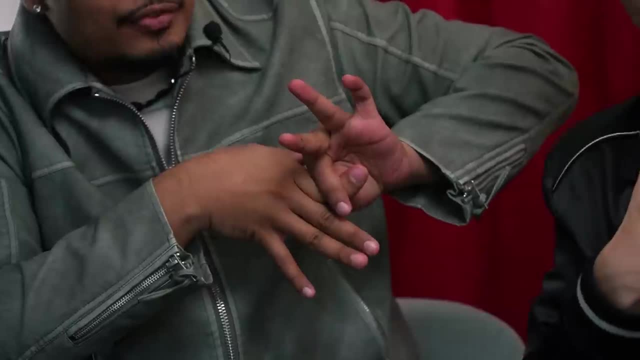 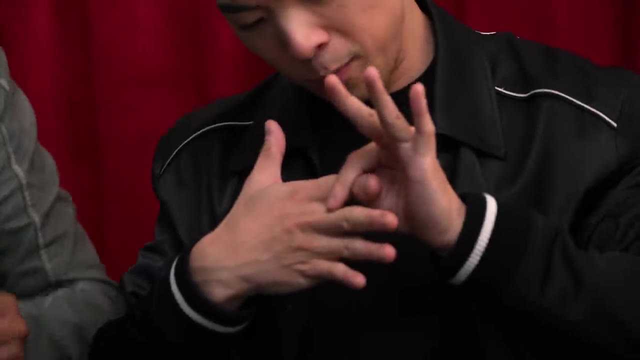 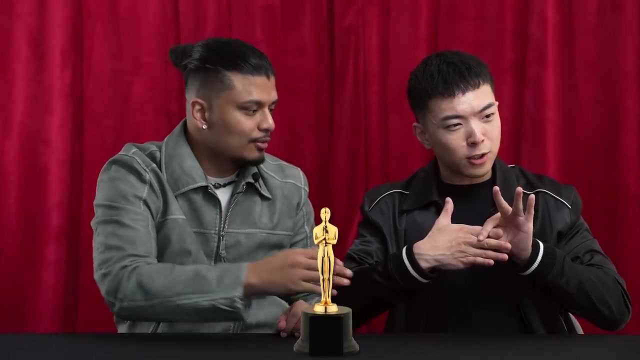 So you're going to maybe do a little bit of bending. You're like, oh, okay, we're going to bend the finger And then you're going to pull, Oh my goodness, Boom. So you go like: That was good, Can we bring his Oscar out now? The Oscar for acting over here. 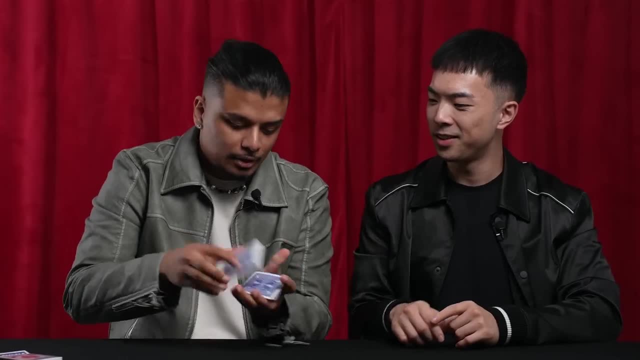 For level 20, we have a card trick. Take a look, Here we go. Watch If you take any card you want. All right, This one. Watch carefully If you take this card. you see right here: Watch If you take. 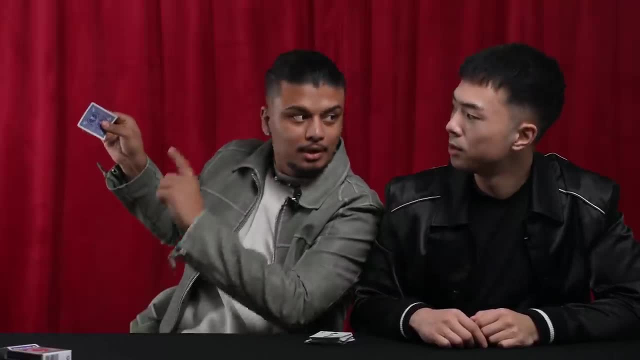 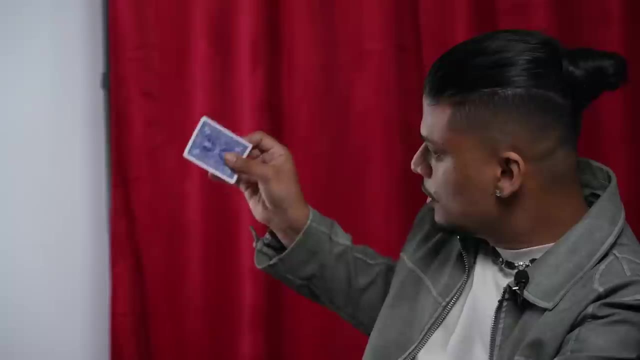 this card? you see right here, Watch. If you take this card, you see right here, Watch. Okay, If you take it, you can actually put it in a different dimension. You can bring it right back, just like that. I'm watching from the side and I still can't see where it went. 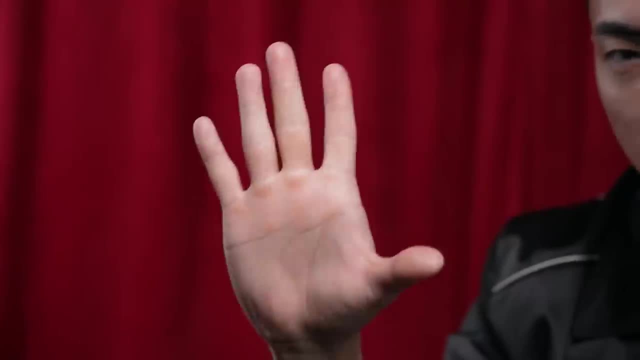 Do you want to learn how that's done? Of course, All right, here we go. So first you're going to do Spider-Man pose and then you put your thumb down like this. What you're going to do is you're going to take your card and that's. 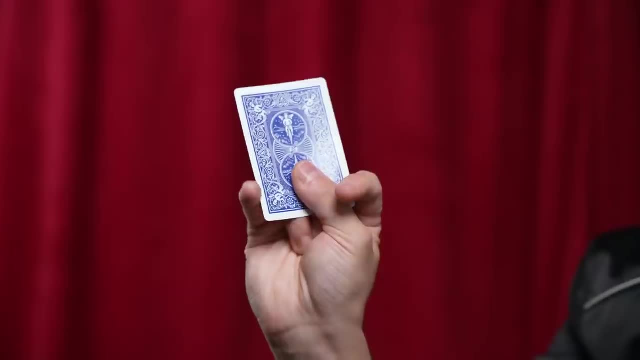 where you're going to hold your card, Right there. Step two: what you're going to do. you take these fingers and you're going to curl around. Now the next part is easy: You just keep your hands closed, but you open your hand. There you go. 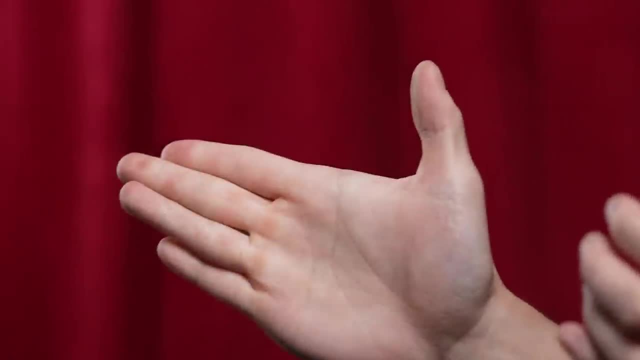 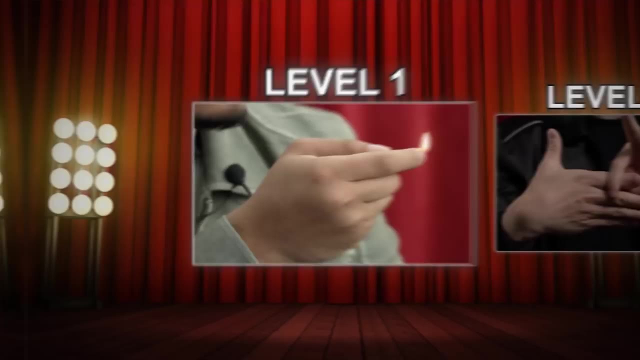 But you got to work on it. You got to work on it. The way you show it less is by holding less of the card- Level 40. This trick will blow your mind. So this trick actually uses a finger ring. I want you to take a look. Make sure there's. 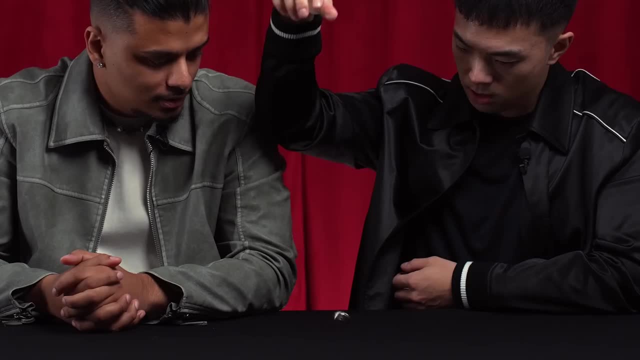 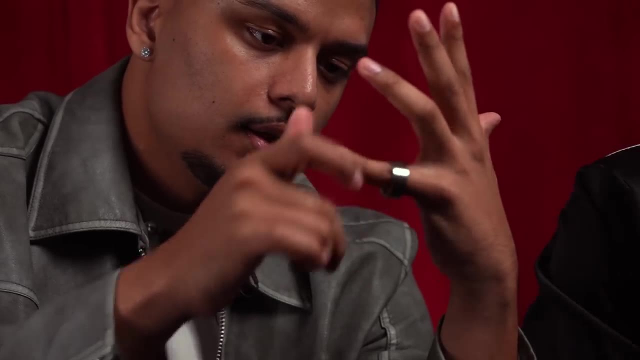 no like slits or cuts or anything like that. It's a real ring. It's real Solid ring. I'm going to take the ring. I'm actually going to put it on my finger like this, on my pinky. You can take a look. 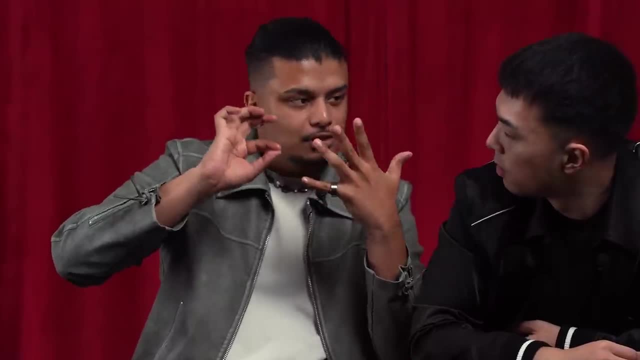 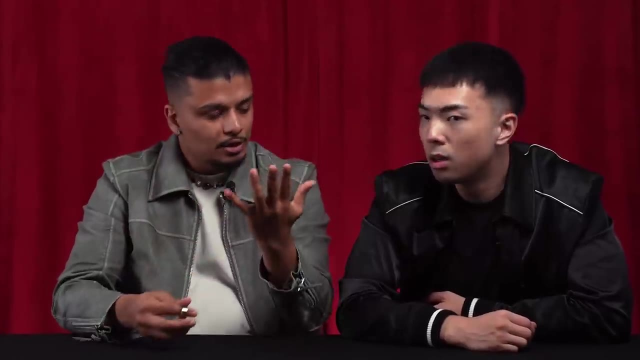 Good, Yes, And try to get solid to pass through solid. Take a look Ready. One, two, three, Just like that You can get the ring to pass right through the finger. No, How'd you do that? You want to learn it. 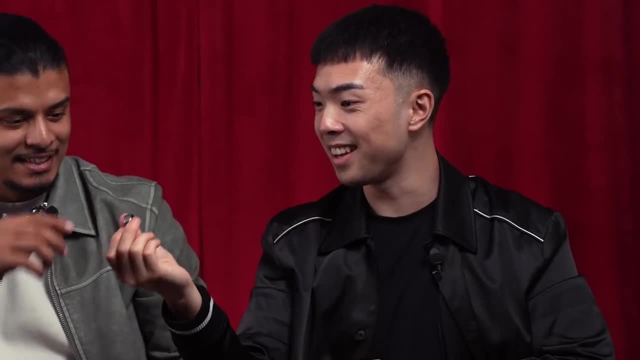 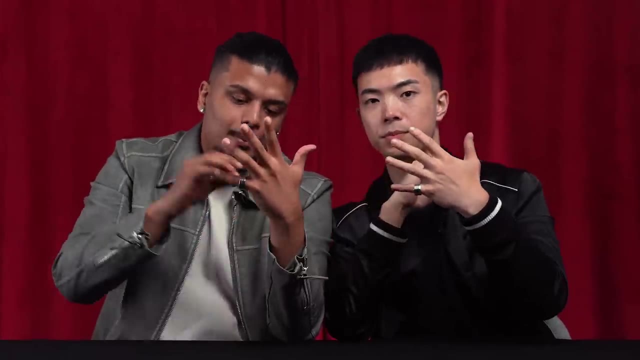 Yeah, This is insane. All right, Here we go. So it's a normal ring. You can use any ring. You put it on your pinky finger like this: Okay, Perfect. Now here's what happened. Okay, You're going to hold it like this: Two fingers on. 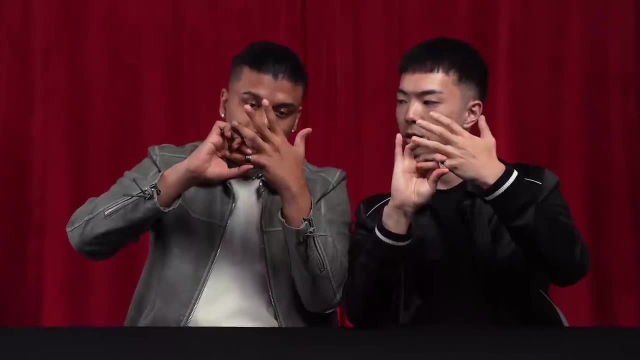 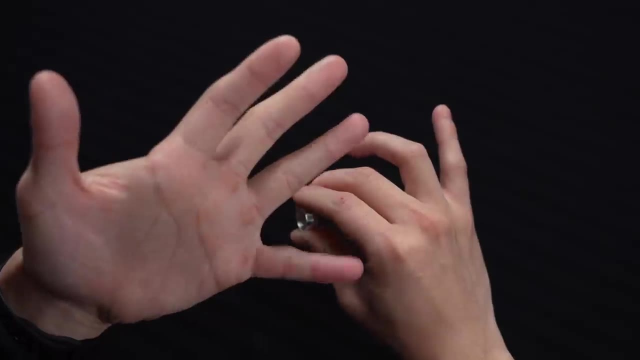 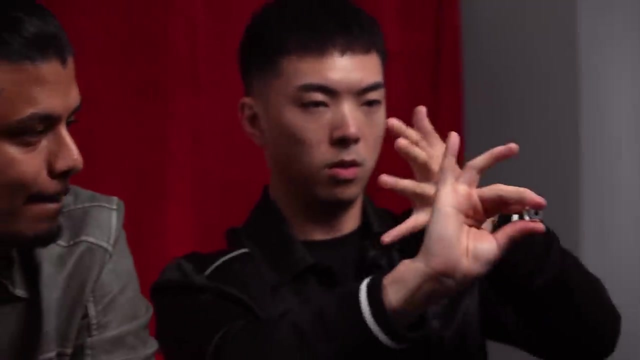 top one and your thumb on the bottom, like this: Okay, And you're going to push straight forward and through. What's going to happen is your finger is just going to naturally glide out of it And you're pushing straight through in one swift motion: One, two, three, Just like that, And you push it right off- Boom. 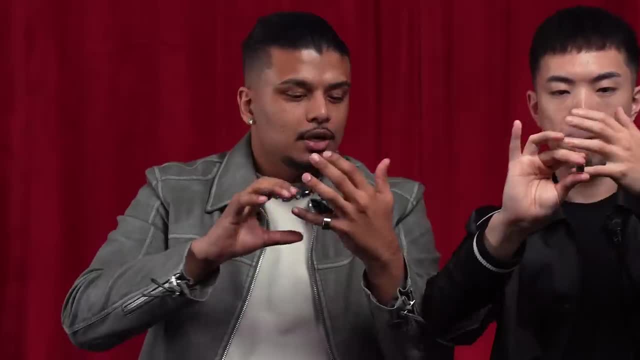 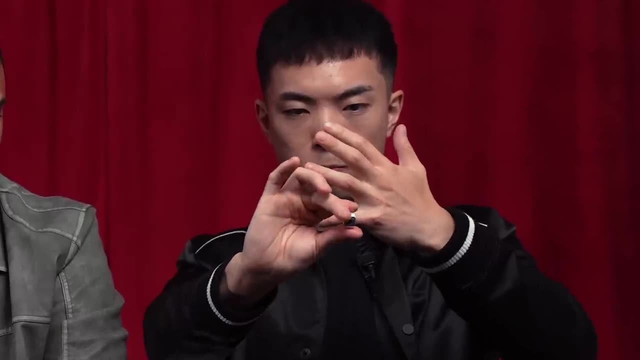 Something like that. And no, Try to control it, because you're like shooting it far too much. You just want to go straight ahead of you. There you go. That was good. That was a good one. That was a good one. 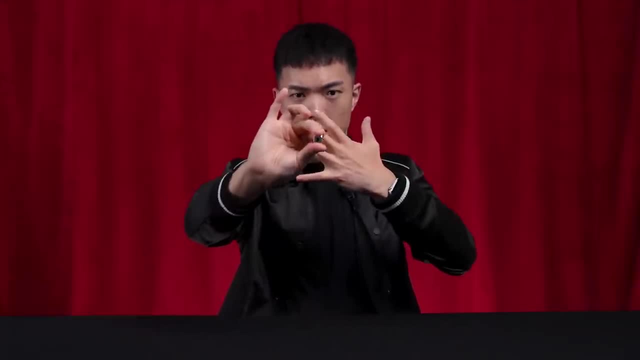 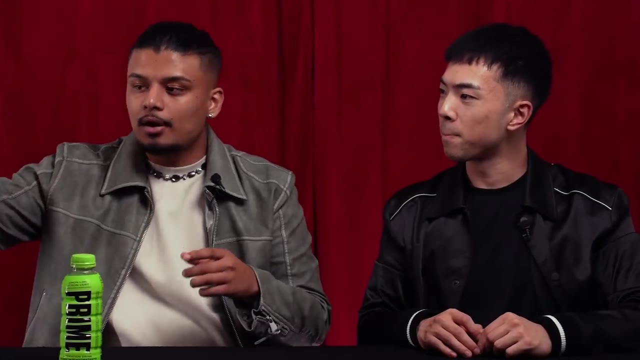 That was good. Now we're halfway through, at level 50.. And this is the vanishing bottle trick. Take a look, We have a prime bottle and we have an empty bag. You can see here We take the bottle, put it inside the bag like this: You. 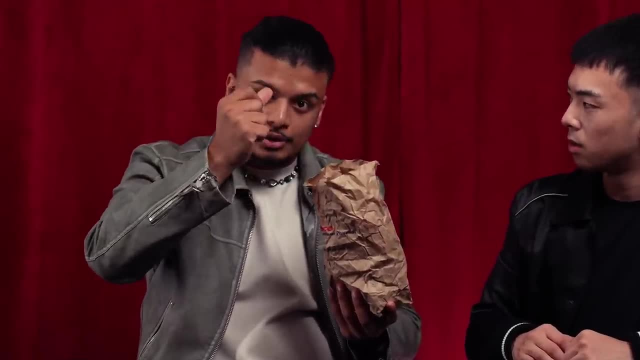 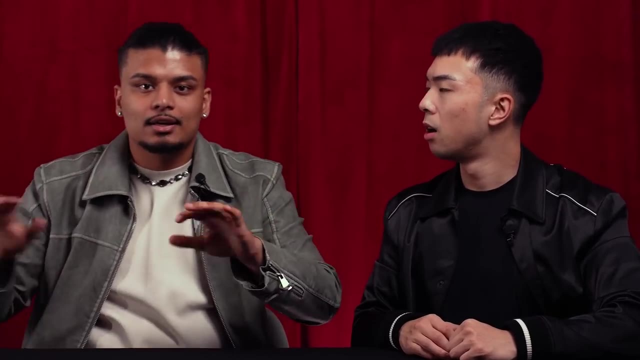 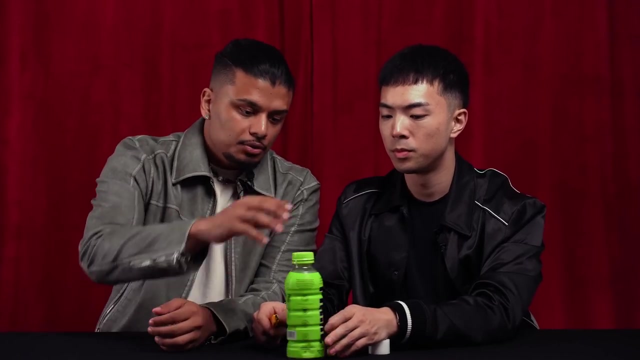 wave over the bag like this and you snap and something crazy happens. Watch The bottle disappears, completely gone, Just like that. For this trick you need a sports drink bottle, A knife and some tape. So once you have all the things that you need, you take the bottle and you want to make sure. 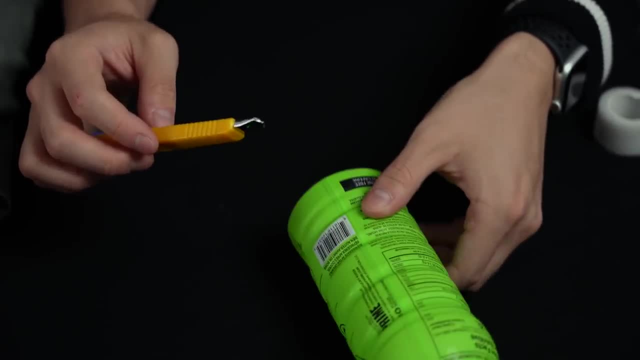 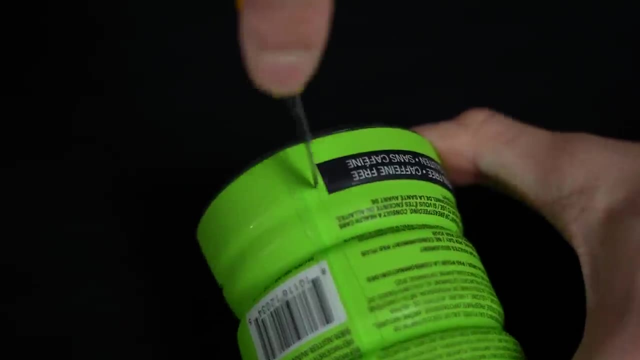 that the logo is facing forward And what you're going to do is you're going to lay it flat down like this And I want you to just slice down the back so that you can cut the wrapper nice and clean down the back. Once you've done this, you want to take the 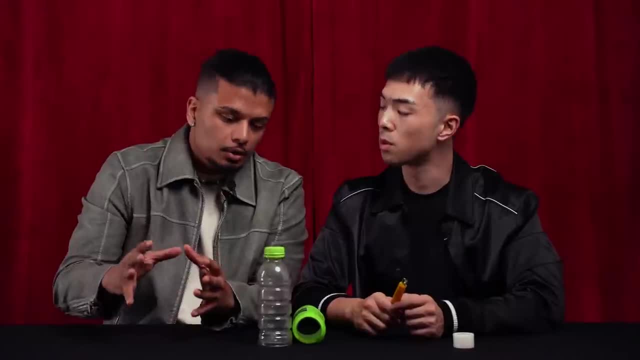 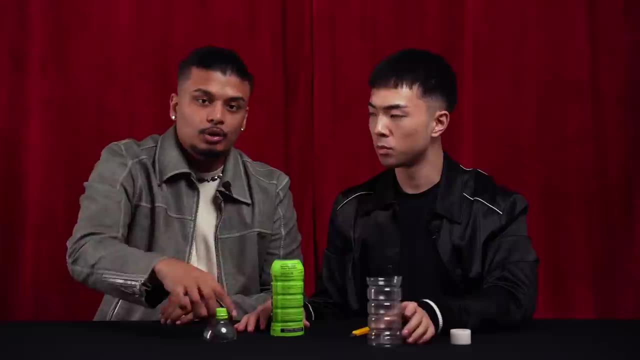 wrapper off and keep it safe, because you're going to need it very, very soon. So now what you want to do is you want to cut off the top portion of the plastic bottle, maybe one or two inches down from the top, So you just have this top portion Once you have your 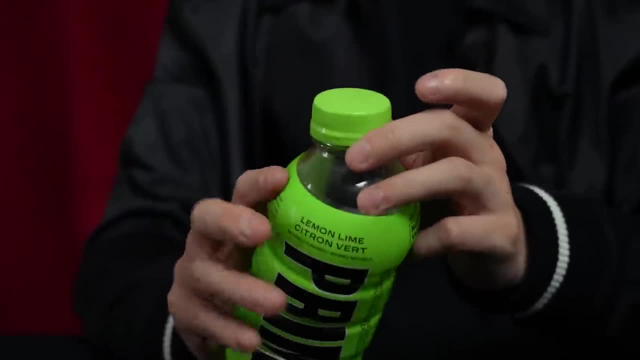 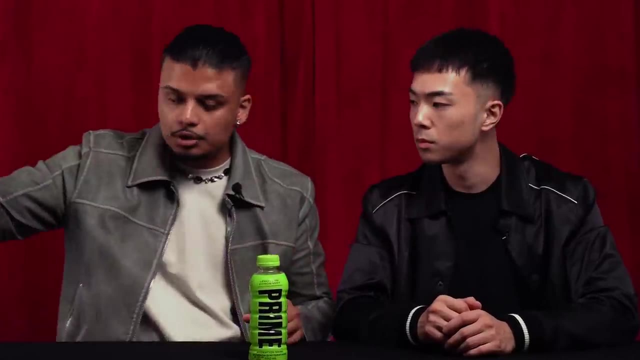 top portion like this. what you're going to do is you're going to take the wrapper and you're going to put it back on and then you're going to tape it on So it looks like the rest of the bottle is there. So, once you've got your shell of a bottle, what you want to do is you want to get an. 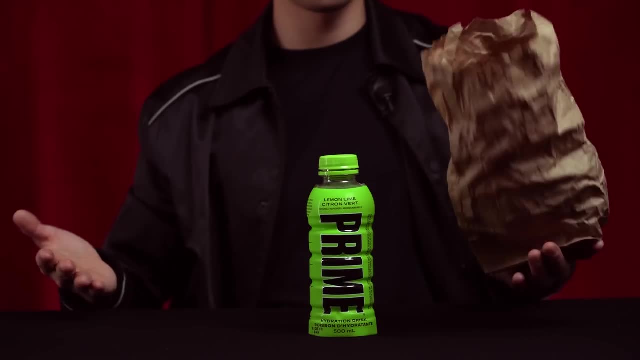 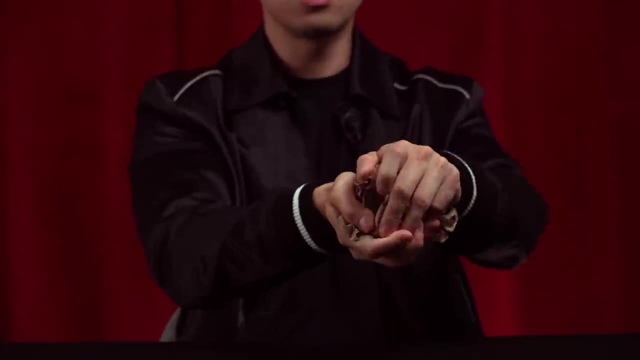 empty paper bag. It can already be crumpled, It could be brand new, It doesn't matter. And what's going to happen is this: You're going to take the bottle, you're going to put it inside and once you're ready, you just smash it, because all you have here, really, 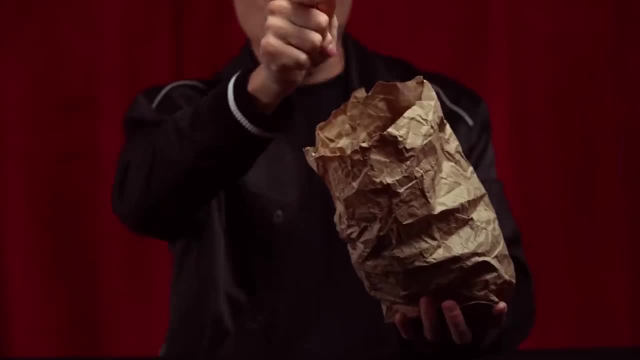 is this much of the bottle. Everything else is just plastic. So when you crumple it, crumple it, This looks like the ball. Correct? This is a genius trick. Shout out to E Katarina for teaching me. 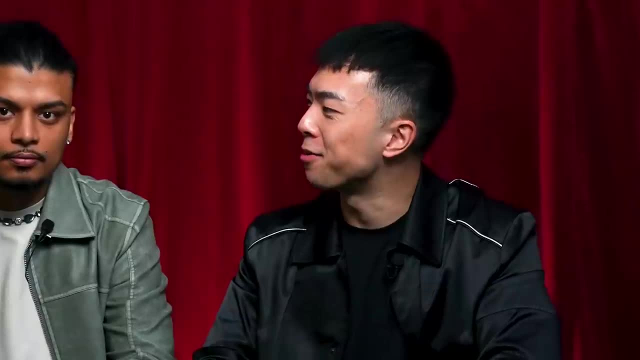 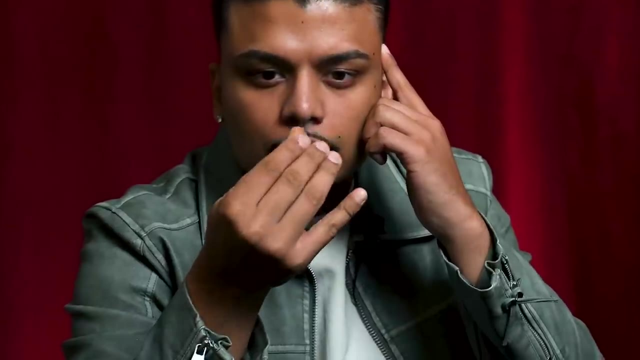 Now it's time for level 60.. What trick do you have for us? Do you know what happens when you focus really hard? What Let me show you. Watch. Oh, You can generate smoke just like that if you focus. Wow. 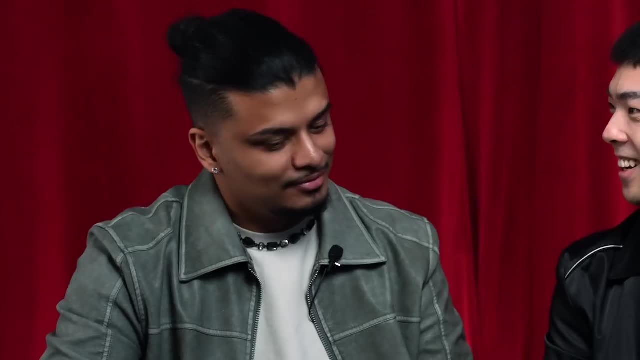 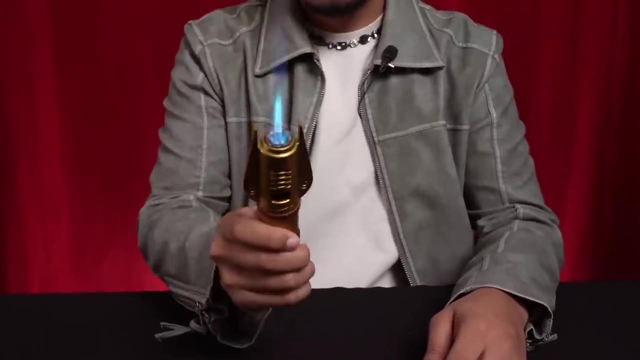 They call it magic fingers. That's what the ladies call. you too, right, All right. So for this trick, we're going to need a ceramic mug, We're going to need a matchbox, We're going to need a lighter, or a torch in this case, And that's all you. 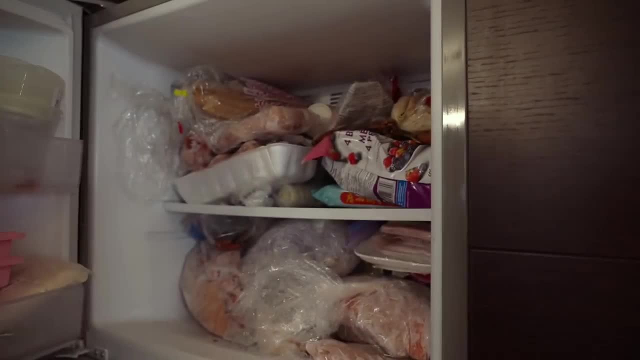 need And we can make this trick happen. First, you need to take your mug and you want to put it inside a freezer, so you can maybe let it sit there for 15, 20 minutes, just so that it gets nice and nice and chilly. Next, 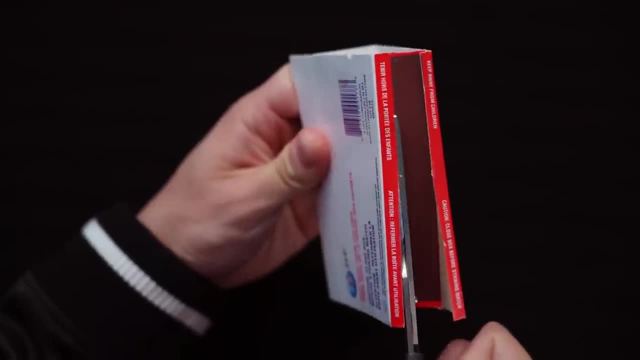 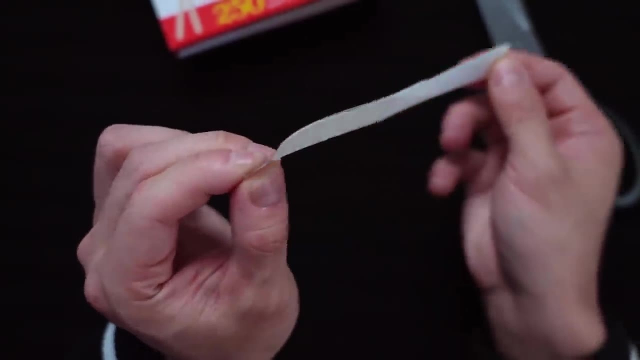 you want to take your matchbox and you want to cut off the striking portion from the matchbox. Then you want to peel the striking layer from the paper so that you're left with just again the striking layer. Next you want to fold it in half, place it on top of your mug, like so, so that the striking 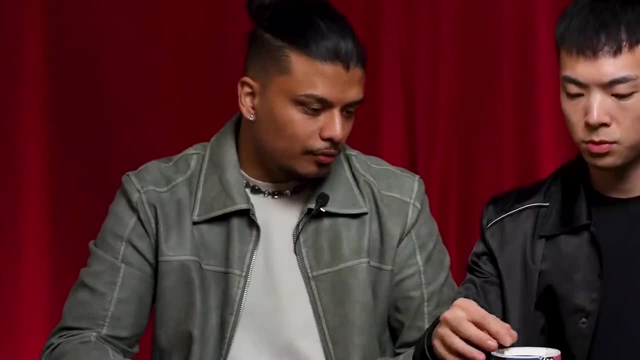 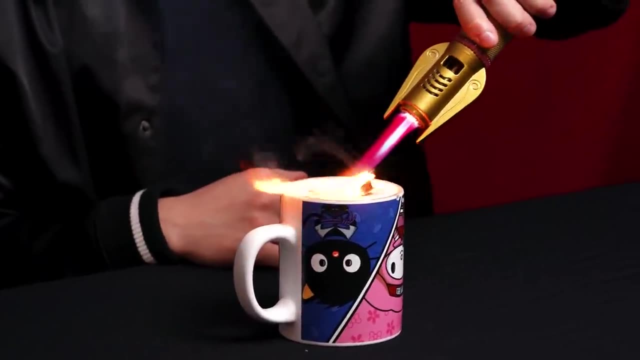 layer is directly on the mug, And then you want to light it on fire. So be very careful with this. As this burns, what's going to happen is the chemical we need is actually going to get stuck onto the cold ceramic mug, And that's what we're going to use for this trick Now. 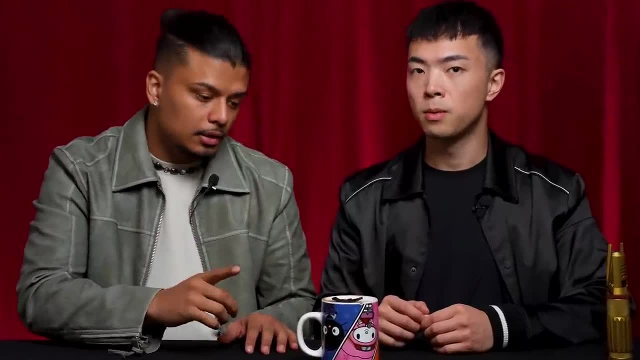 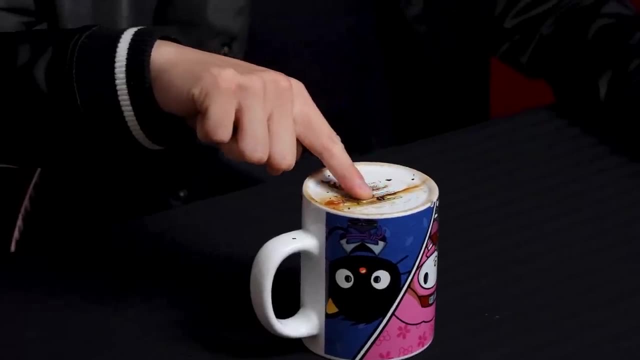 you want to make sure that you wait until this is completely cooled down before you go ahead and use it. Now you want to take one or two fingers and you want to take a nice big scoop of the goo that's left over on the cup, Just like that, And now you just have to rub your fingers. 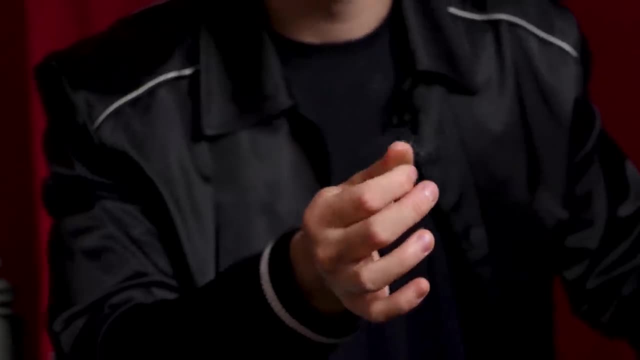 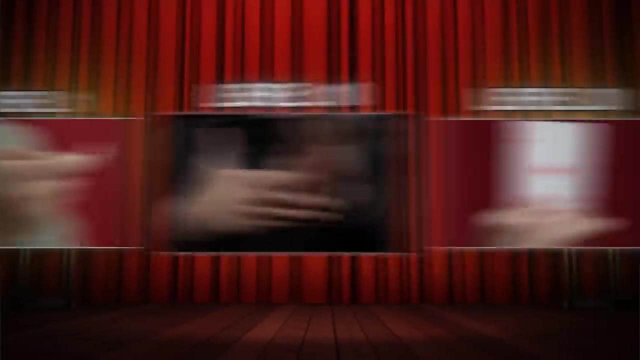 together. Boom, There you go. You get smoke. Oh Oh, This is so cool. Now let's see what other tricks you have. Next is level 70.. I'm going to do something that will break the laws of physics. Watch carefully If you take this glass. I'm going. 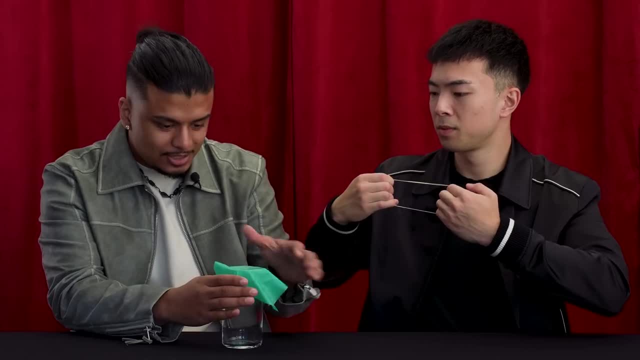 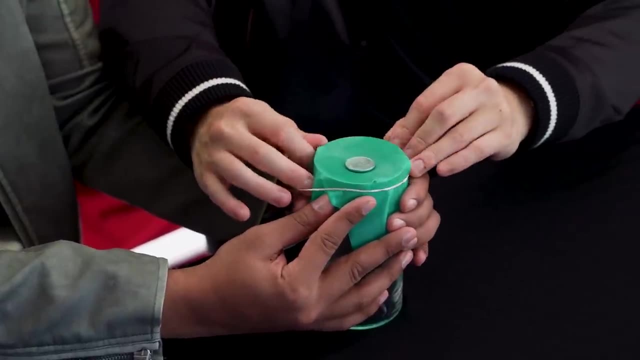 to put this on top like this: Can you please take that rubber band and can you seal it off on every single side? Go ahead, Perfect Watch. I want you to take a finger like this: Hold it out, Perfect, Good choice. I want you to point it down like this: I want you. 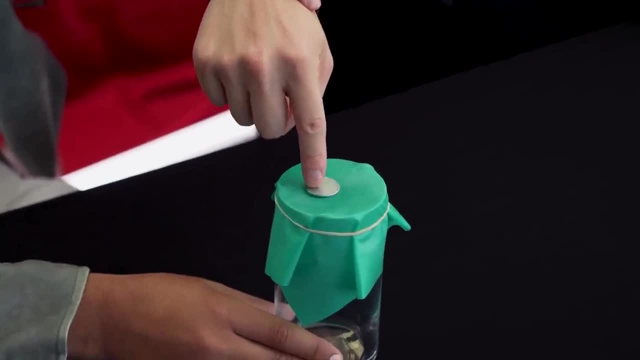 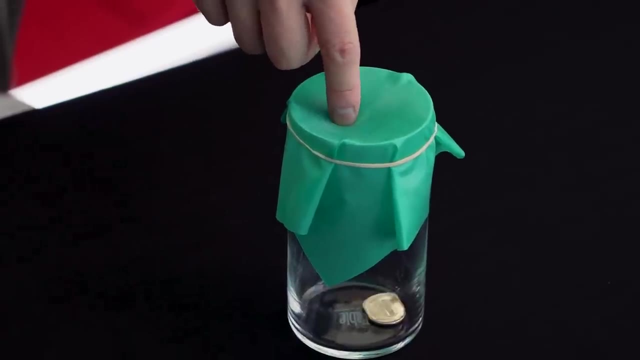 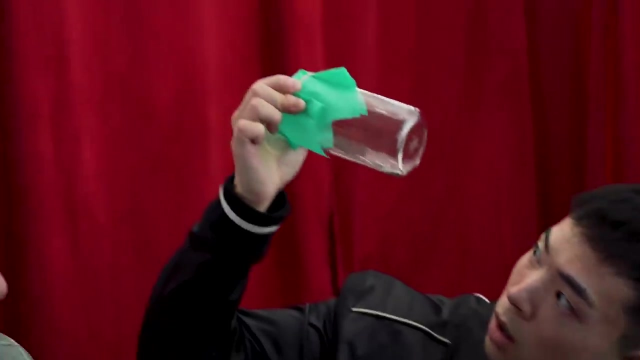 to slowly rub the coin just slightly. Okay, Just a little bit, Just like that, Perfect. And I want you to now push down onto the coin. Go ahead, Push, Push, Push. Just like that. You can get the coin to go all the way through. Watch, You, take a look. 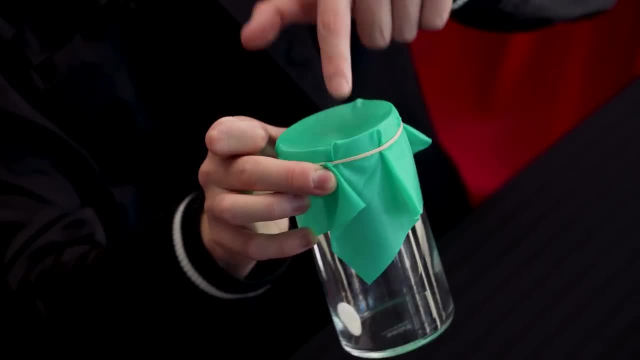 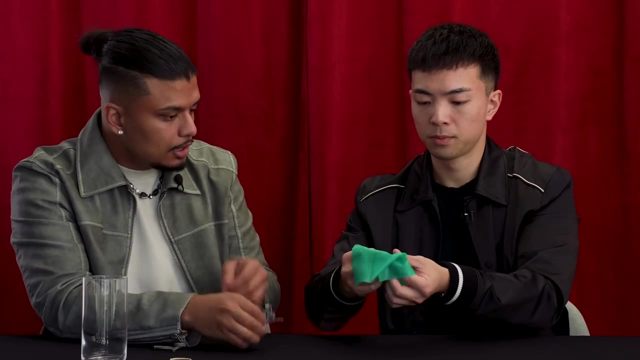 There's like a little mark where the coin went through, but there's no hole. Please teach me. All right, Here we go. So this is how this works. We use a really thin but stretchy sheet of rubber. Take the rubber, stretch it out. There you go. Yep, Yep, I'm going to get a. 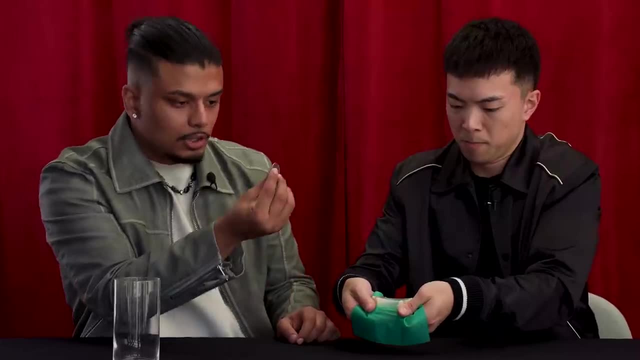 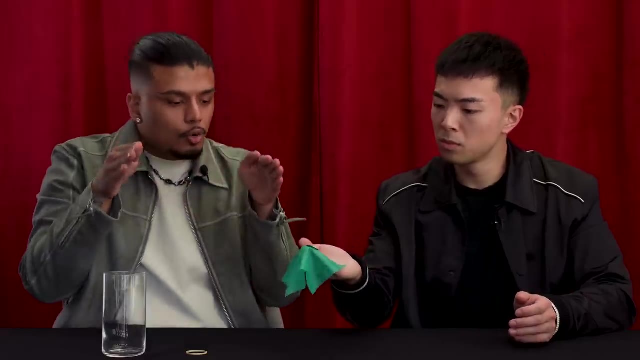 nice stretch. So once you get the rubber stretched out like this, you take a coin from underneath, you push it straight up like this, and then you let go and the rubber is stretching over the coin and it makes it look like it's on top right now. Isn't that crazy. 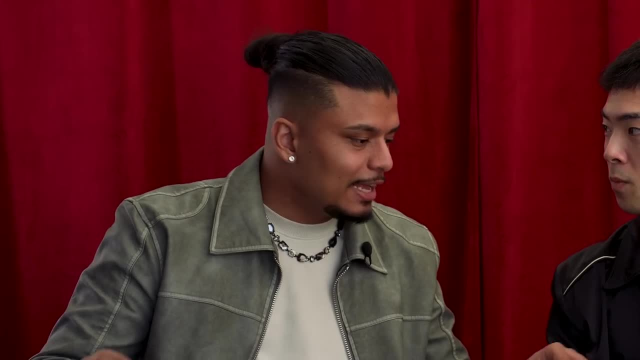 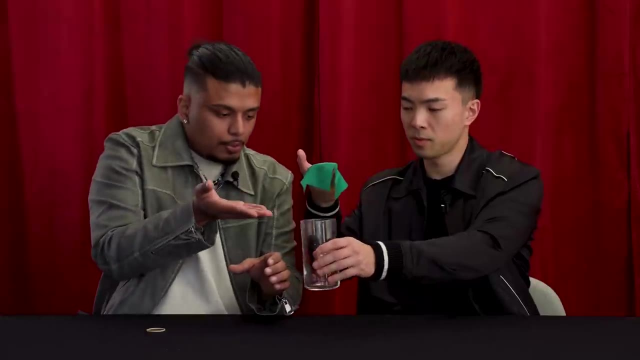 Yeah, Look at this. That is so sick. So the next part is making it real magic. Okay, Take the cup with your other hand. Okay, You can show the cup as well if you'd like, and you carefully just place this on. 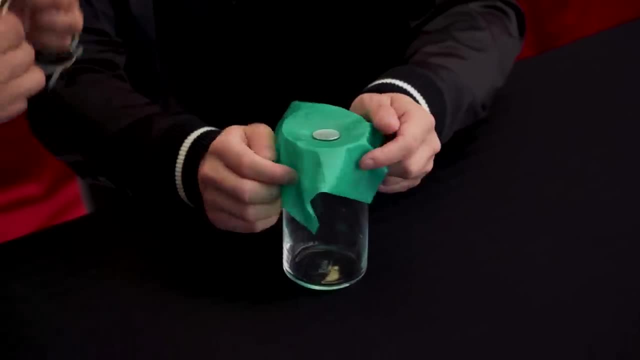 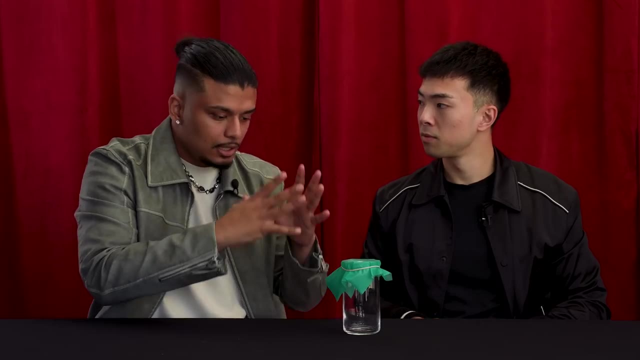 top. Perfect, Just like that, And you can ask someone to help you with this. The next part: just take any rubber band and just place it on top like this, covering it on every single side, And that is basically the entire setup for this trick. The rest is all presentation. 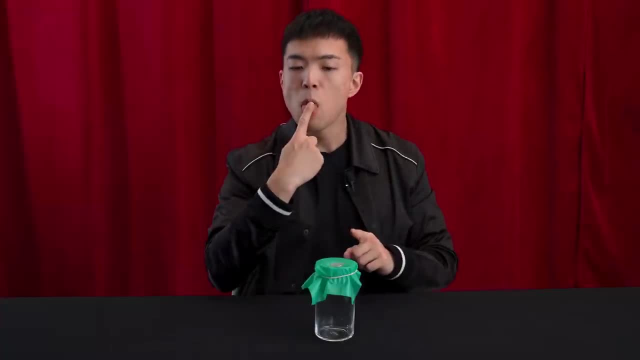 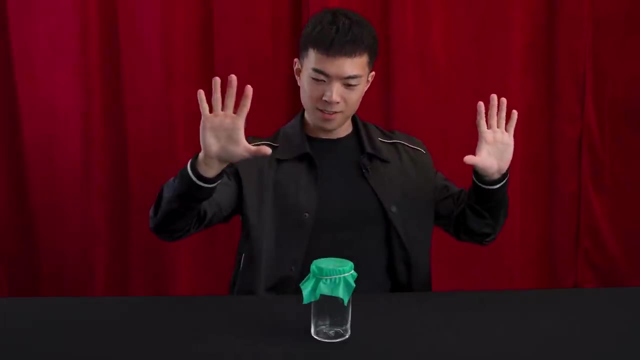 You can tell someone: take your finger, You want to heat up the coin, You want to do whatever you'd like, and push it straight down and something magical will happen. Take a look, Boom, Wow, There you go. And then you can show it off. You can say: look, there's no hole, There's. 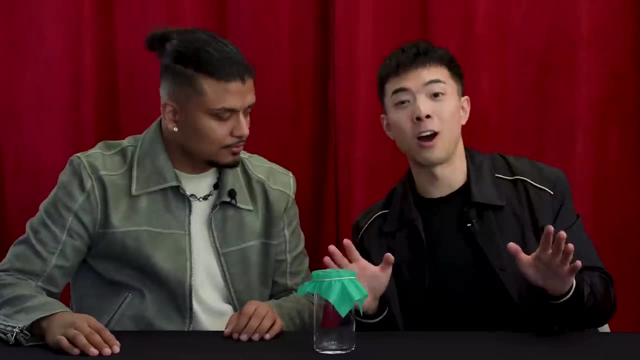 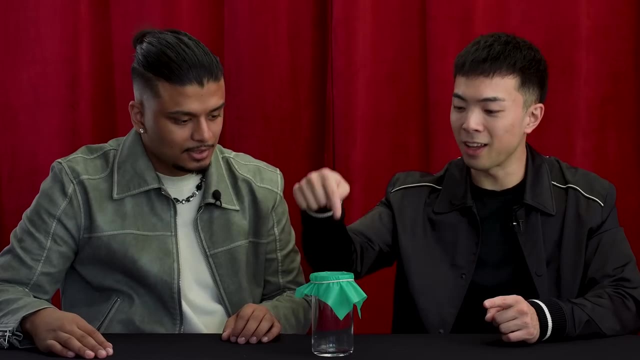 no, nothing You're done at this point. They can look at this as much as they want As an audience member. if I didn't know the trick and what was happening here, like this motion just felt normal, right. Yeah, It just felt like the coin actually. 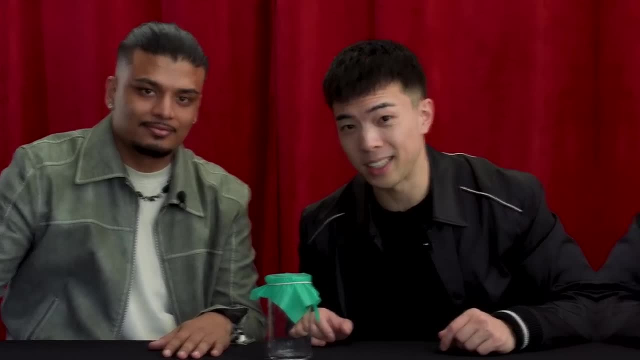 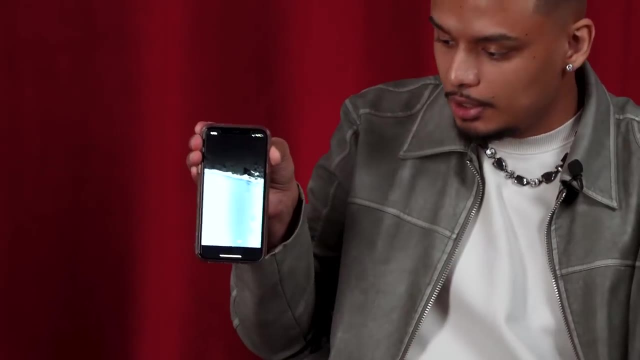 went through the rubber. Wow, Now onto the next trick, Level 80.. Hafu, I heard you were a little thirsty. I'm always thirsty. Okay, Let's fix that. You see, there's liquid on the screen. What we can do is use a little bit of magic to make. 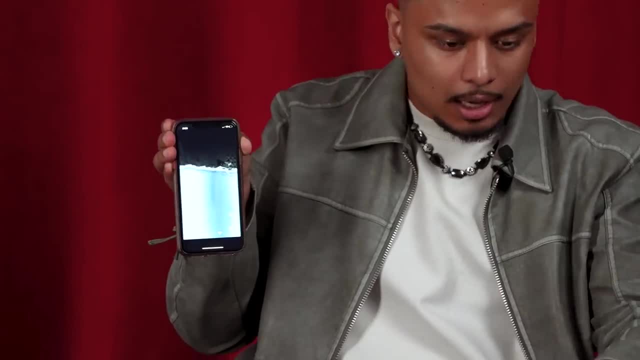 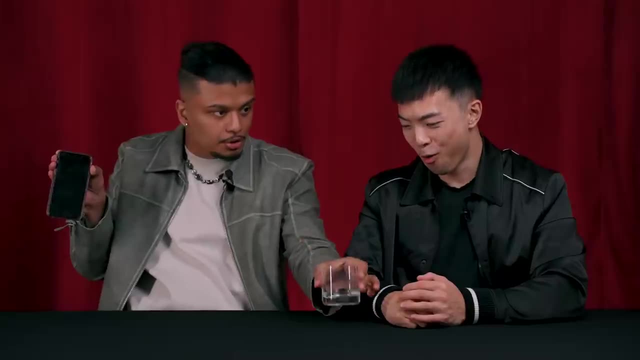 something crazy happen. Watch, You do this, you get a cup. Okay, Watch, We're also about to have a Jesus moment. You can actually get some water for you to drink. my friend, That is for you. Is this real? 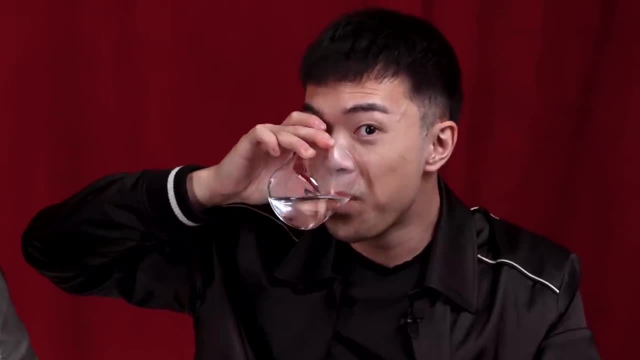 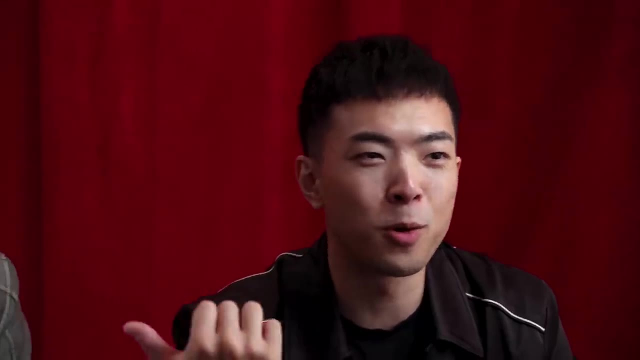 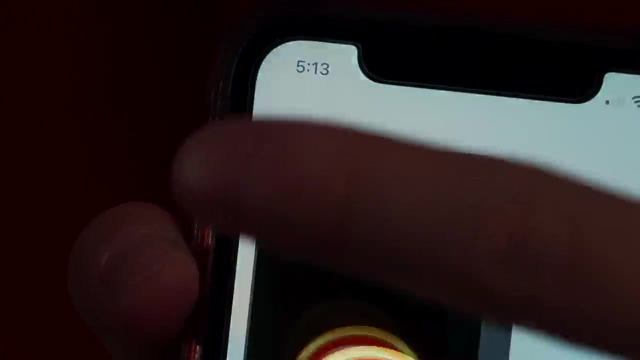 It is real, Absolutely. That is real water, Real water Damn. That's like a iPhone 20- future right. So what you need for this is an app. It's called iBeer Free. It's not free, You got. 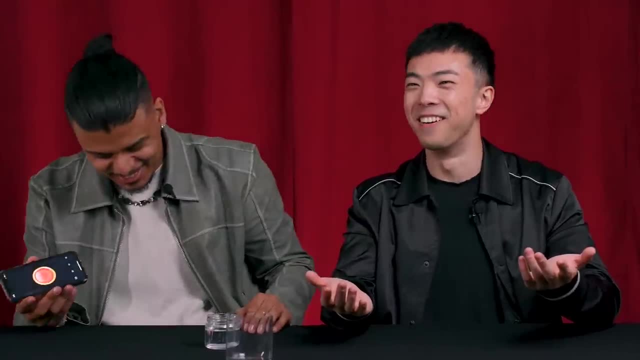 to pay for it. But once you get the app, That's such a scam. What? Once you get the app, you have to go and change it to water, because initially it starts with beer, but you change it to water, Got it. 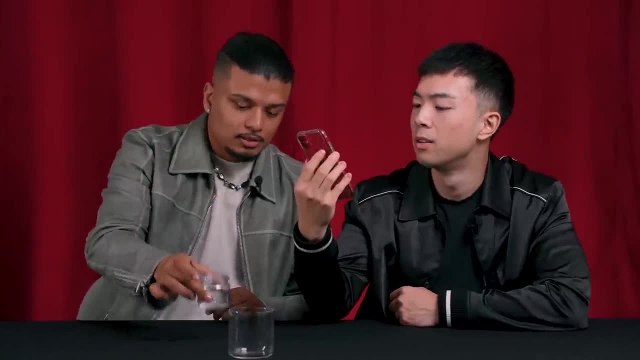 Yeah, Perfect. So that's step one. So the next step is: you need one of these. You need a little cup, a little jar, It could be anything, It's just something that can hold a little bit of water. You want to hold your hand like this. 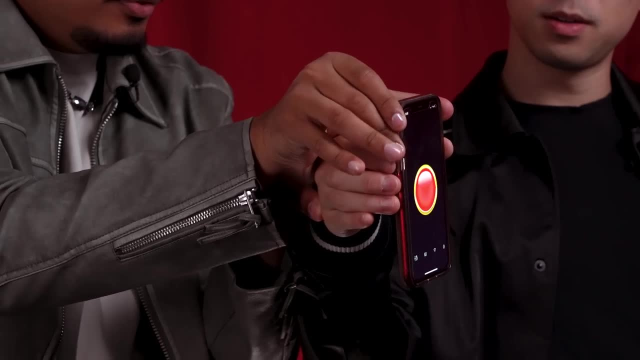 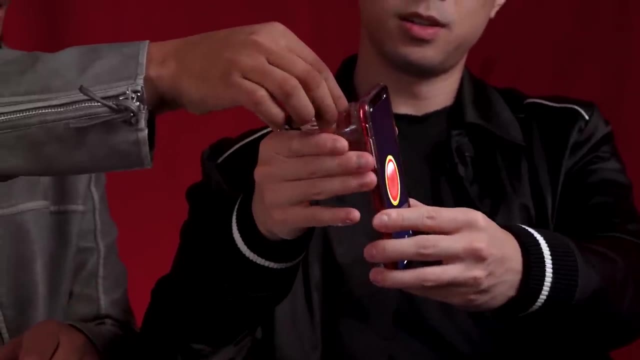 Like this, Yeah. So what's going to happen is: this is going to be at your very fingertips, like that, And this is going to go right behind like this, You want to hold it? Yeah, Just a little bit like that, Perfect. And so when you want to start the trick, what you do is you hit. 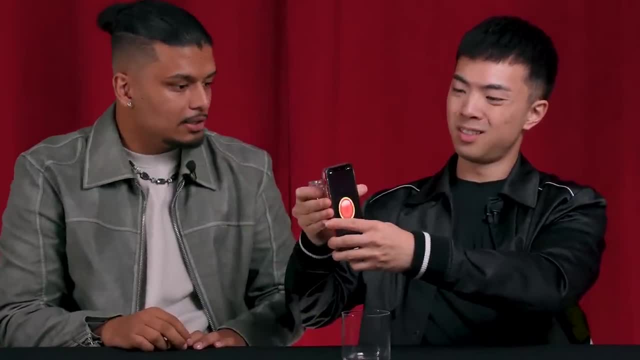 the red button. Not yet. It's not yet. And you grab the bottle like this or the cup like that, Okay, And then you just pour to the left, That's all it is. So you hit the button, Yep, Go. 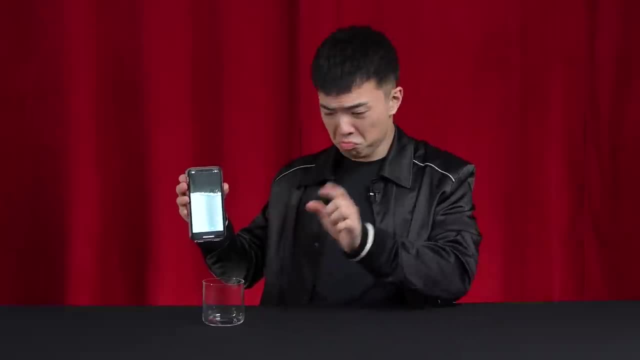 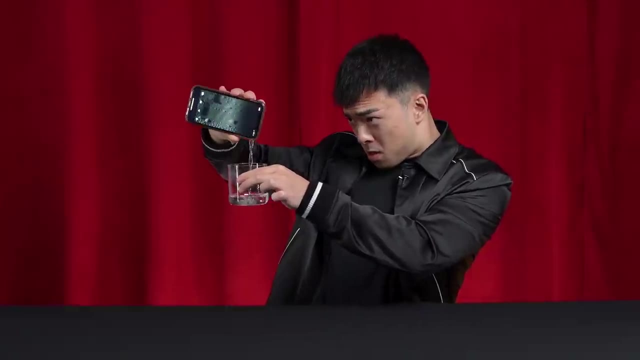 ahead And you show it a little bit, Shake it, Hold on, Yep, It fills up. You shake it left and right a little, It's like that, And when you're ready you just take it and you pour it and you let the water fall, Go And lock the screen. Boom, Just like that There. 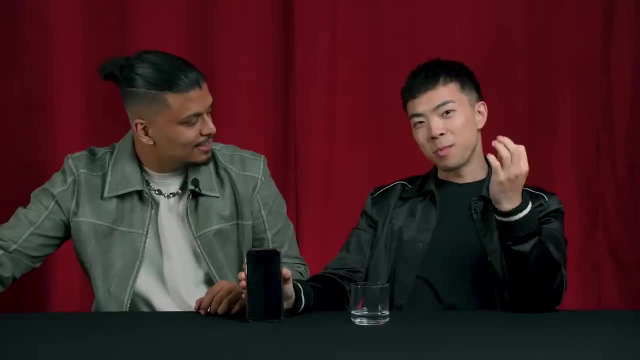 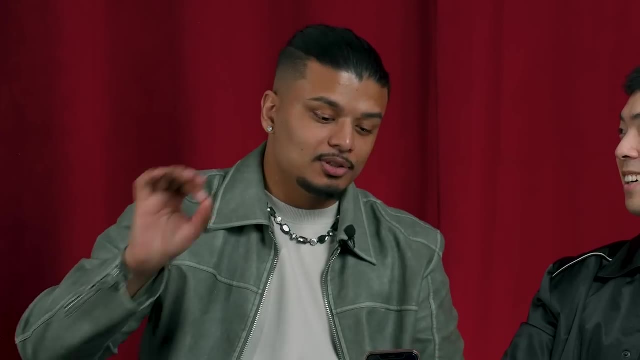 you go. You just made water appear from a phone. Wow, Sometimes magic before you see it seems so complex, but once it's revealed it's like so simple. But sometimes it's the most simple things that look simple. It looks so amazing. Level 90.. This will be one of the hardest tricks, right? 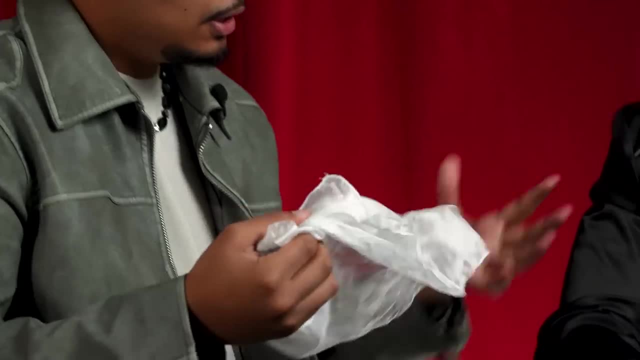 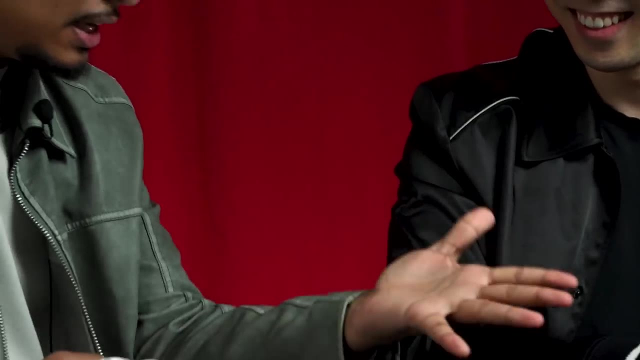 100%. It uses this right here. It's a silk, and it uses my hand here. Look, take a look. Nothing on my hand. There you go, But watch carefully though. Watch this hand. There's a little soft spot you can create. It's a little hole. Can you see that? The hole right? 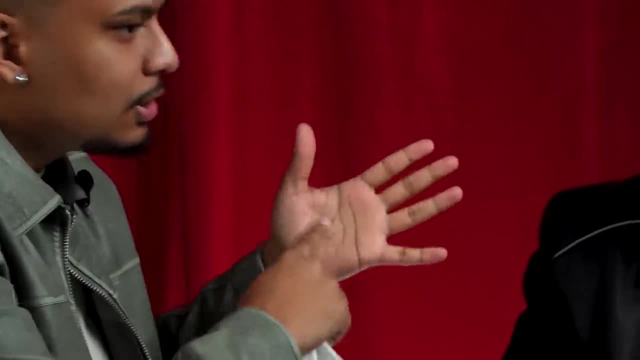 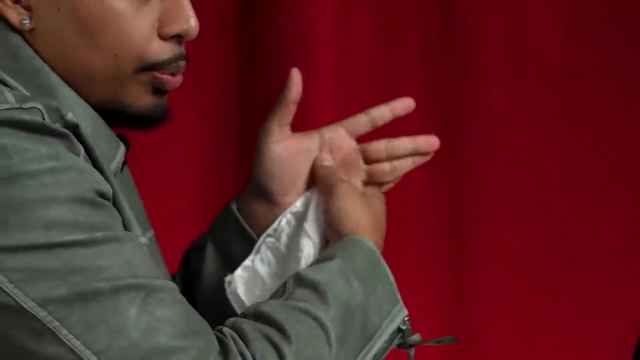 there. What are you talking about? There's no hole Watch. You got to rub it a couple of times and then just give it a little push and crazy thing can happen. I think that was it. I think I felt it. I opened the hole because now what I can do is I can actually get the silk to start. 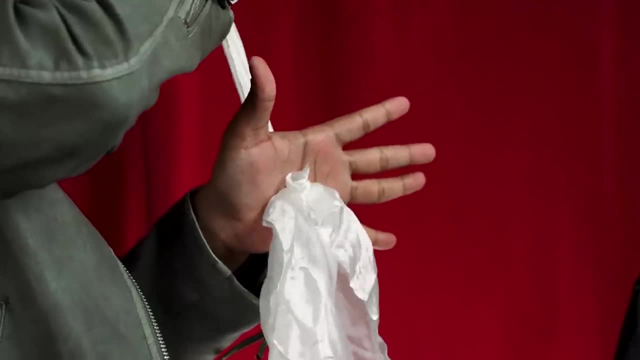 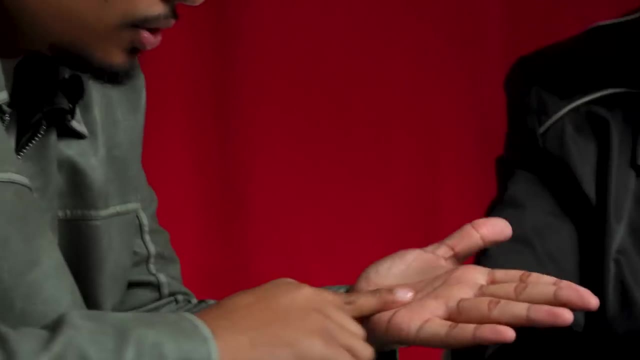 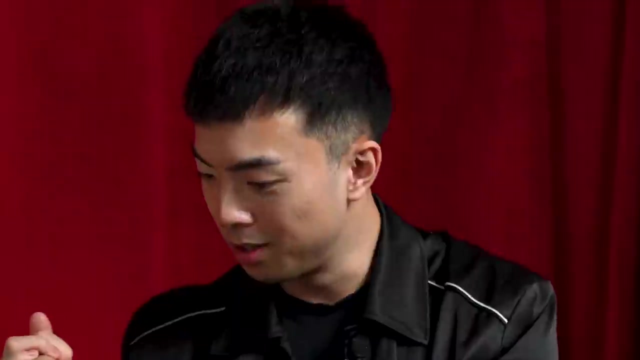 going straight through the hole through your hand to the other side, just like that. And when you want to close the hole, you just take it out and you just rub it like this and it closes completely. Take a look, Dude, does it hurt. 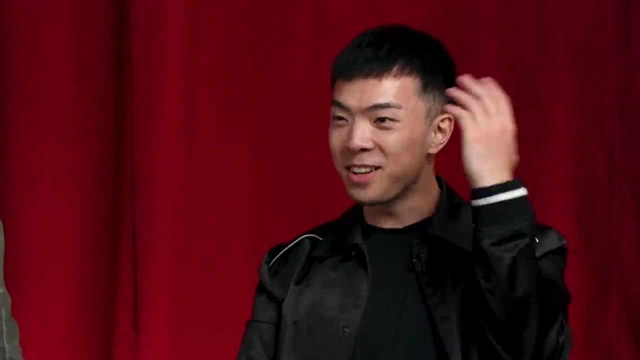 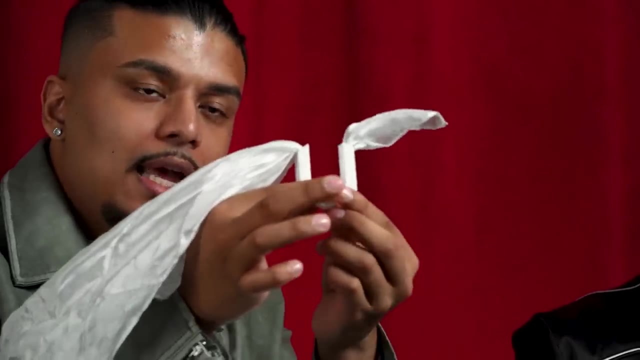 I don't feel a thing. That's insane. That's one of the craziest tricks I've ever seen. How this works is very simple. Obviously, the handkerchief is going through one end and it is coming out the other. This 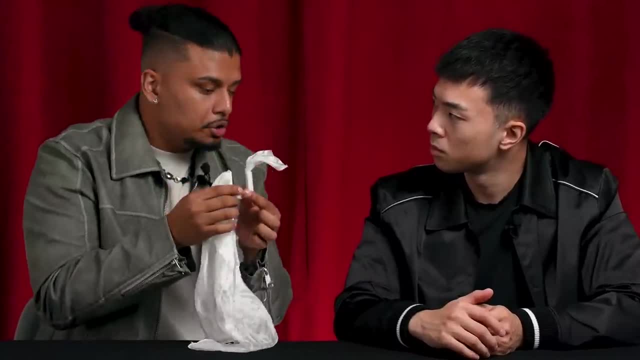 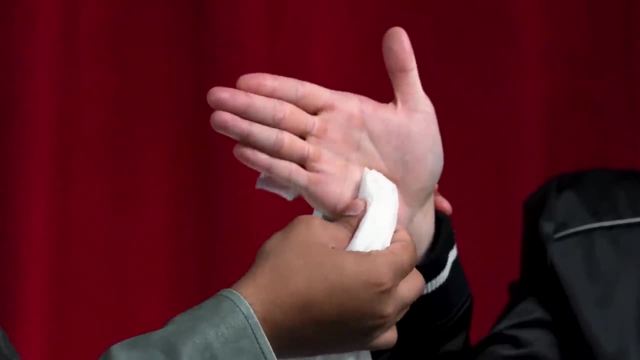 is what allows you to get that illusion of it going through your hand? I'll show you. Can you hold your hand out like this: Okay, Perfect. What happens is this piece goes like this: It gets inserted into your hand like this: Okay, And so what happens is, if you can take your other hand and you pull it. 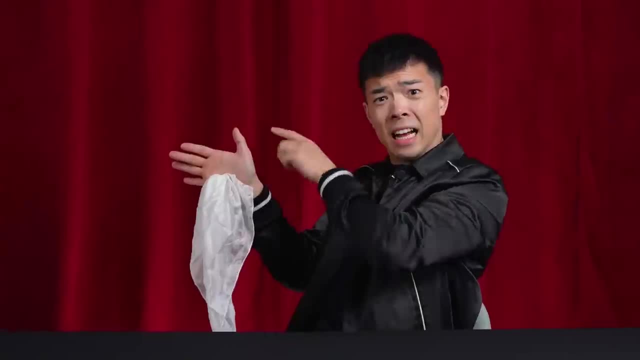 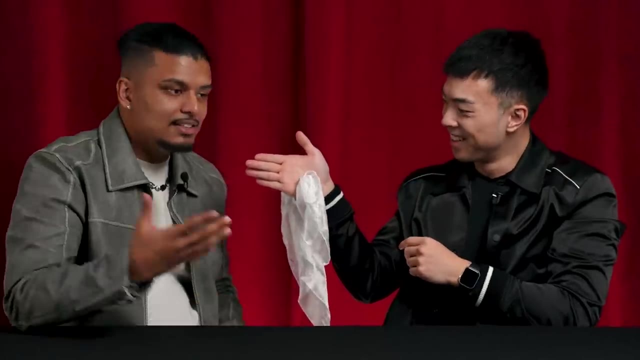 actually looks like the silk is going through your hand to the other side, just like that. This is cool And that's it. It looks so real And when you're done you can use your other hand to just grab it from the bottom. 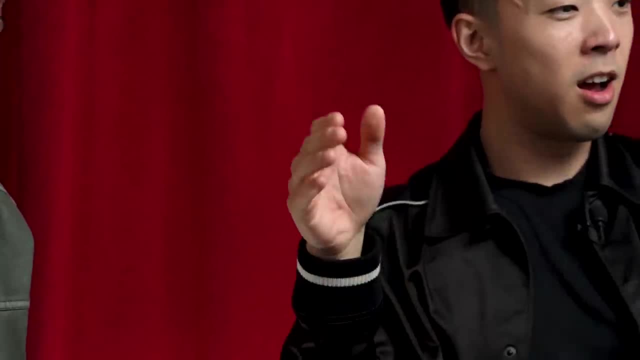 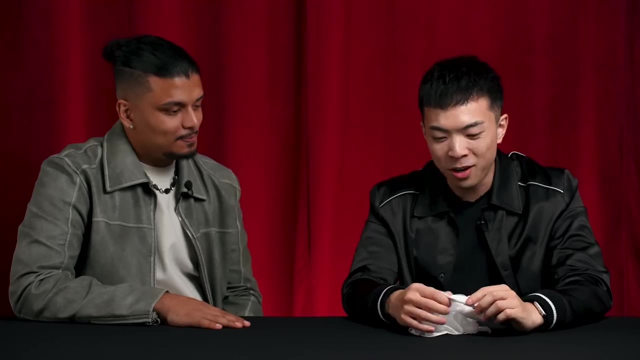 And then you go like grab it- Yes, Just like that. and grab it, Boom, There you go, Done, Just like that, That's magic. Wow, Magic is so deceiving bro. So like what do you think differentiates a good magician? 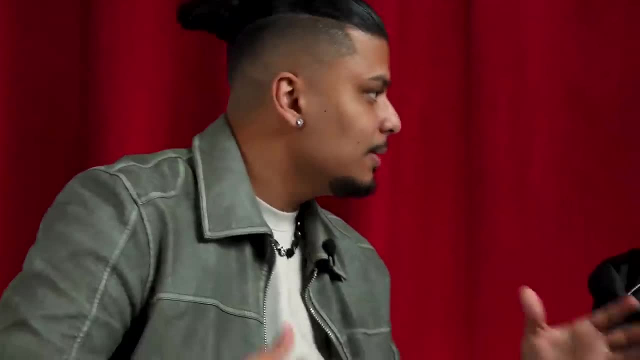 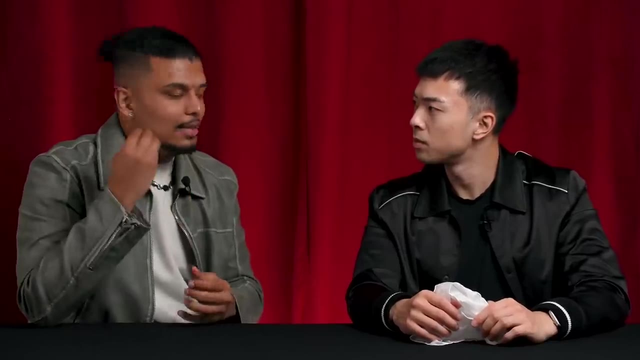 from a bad magician. then It is the presentation, Because, at the end of the day, magic is sleight of hand. It is things that can be learned, But what makes it really powerful is the ability to create a magic trick, And what makes it really powerful is the way you present it and the way you're. 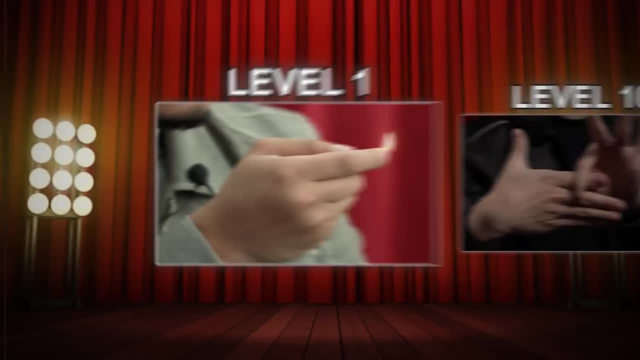 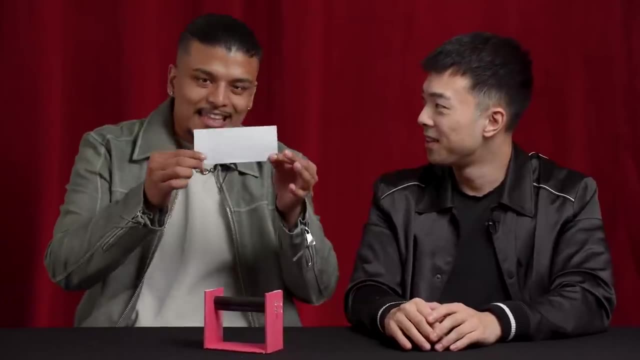 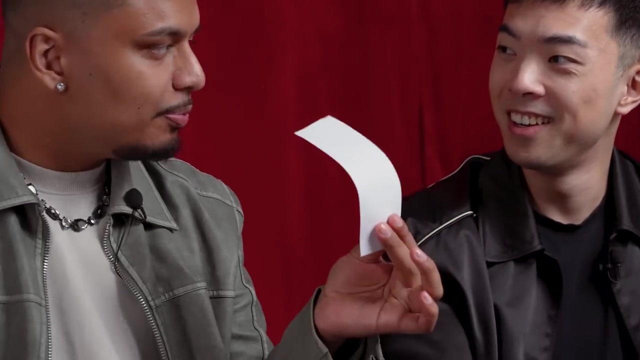 able to deliver a simple magic trick to make it seem so impossible. And now it's time for level 100.. What trick do you have for us, Savio? This is called the infinite money glitch. Ooh, I like money. Are you ready? So what you need for this is a piece of paper. 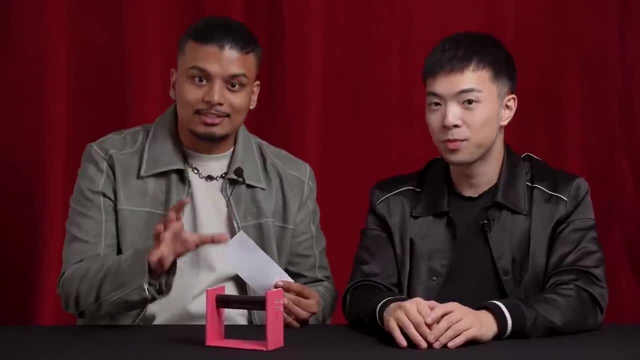 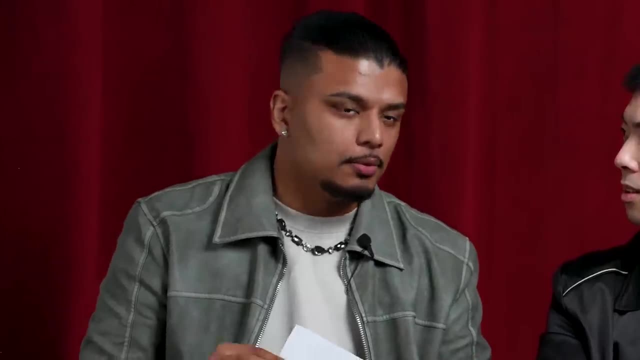 Yeah, And this money printer. I made this with things that I found in my house, But due to the nature of this effect, I cannot reveal how this works. What do you mean? I might get in trouble With who The naughty?